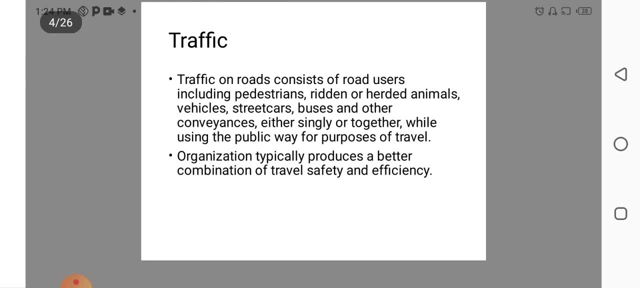 What is traffic? Traffic on road consists of road users, include pedestrian, ride-in or other animals, vehicle, streetcar, buses, other conveyors, either singly or together with using publicways for purpose of travel, Organization typically produces a better combination of traffic on roads. 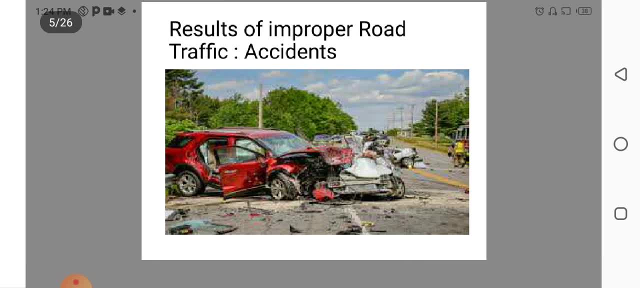 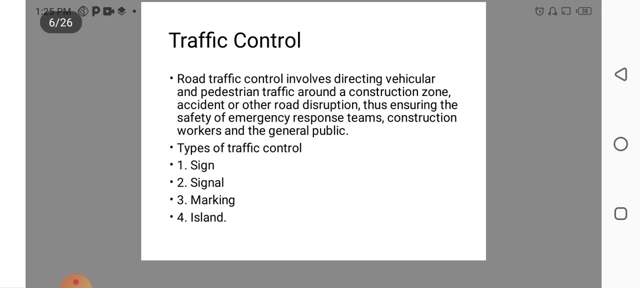 It is a combination of traffic safety and efficiency. What is the results of traffic on road traffic? You will be seeing accidents. So for better traffic on road traffic, we need traffic controls. What is traffic controls Involves directing vehicular and pedestrian traffic. 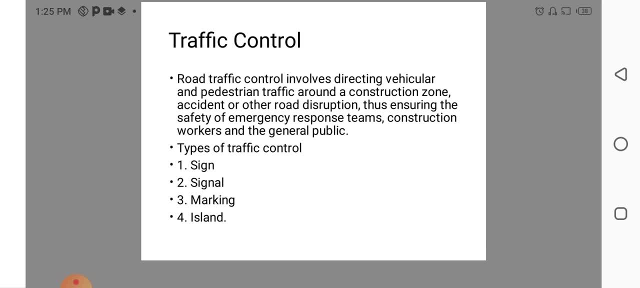 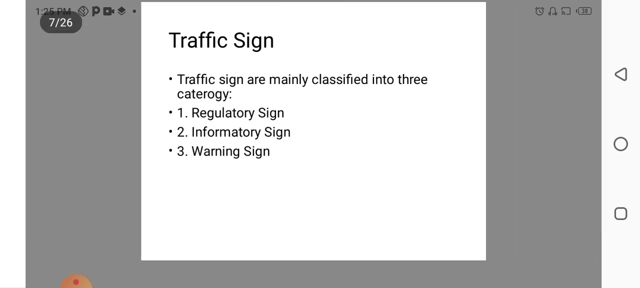 According to the construction zone, accident or other road disruptions, thus ensuring the safety of emergency response team, construction workers and general publics. Now I'll be talking about traffic controls types, such as sign signal marking island. Here, traffic sign is divided into three types. 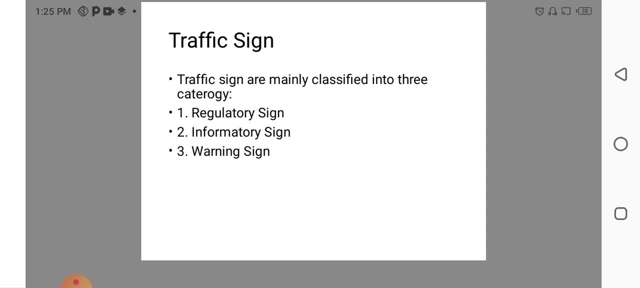 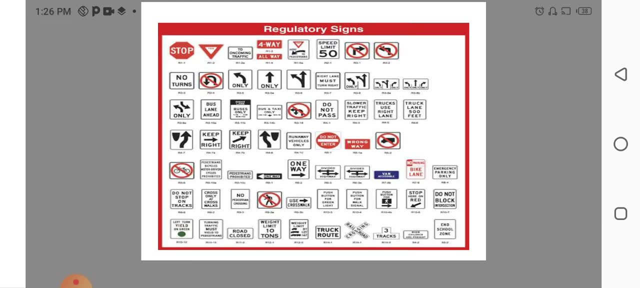 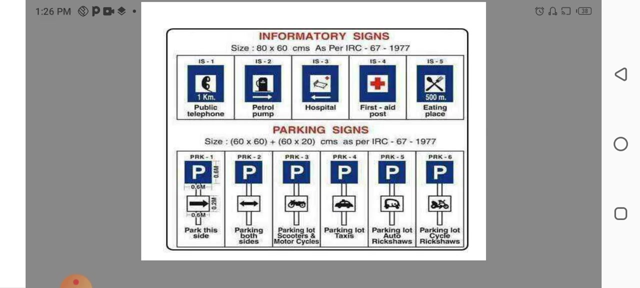 Regulatory sign- informatory sign- warning sign. Here you can see the regulatory signs. It is a mandatory sign, compulsory for all road users to follow. Informatory signs give information about some of the road traffic. Here you can see the regulatory signs. It is mandatory sign, compulsory for all road users to follow. 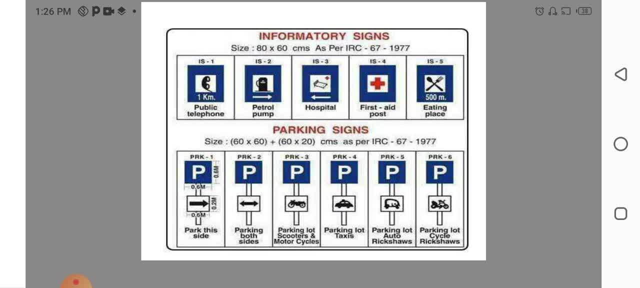 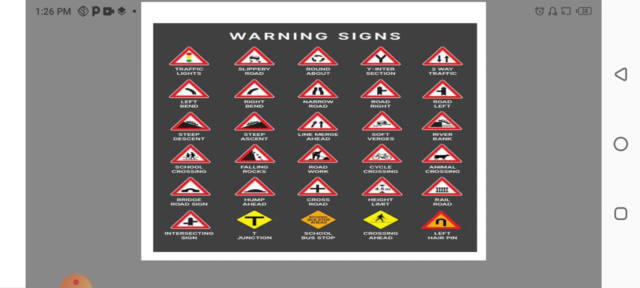 some of the public, private buildings: parking signs, petrol pumps, hospitals, first aid post, eating places, public telephones, etc. warning signs. gives warning to the users in the form of traffic light or in the form of signs. here are the some of the warning shine soon. now I'll be talking about traffic. 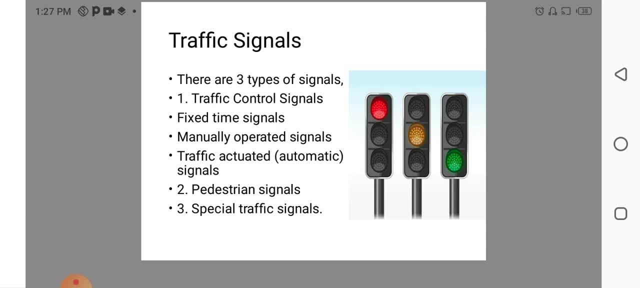 signals. signal are basically divided into three types: traffic control signals, fixed-time or manual operated signal. second one is automatic: automatic here in the second category will. it is divided into pedestrian sign and spatial traffic signals. we will be discussing one by one what is fixed time. fixed time. 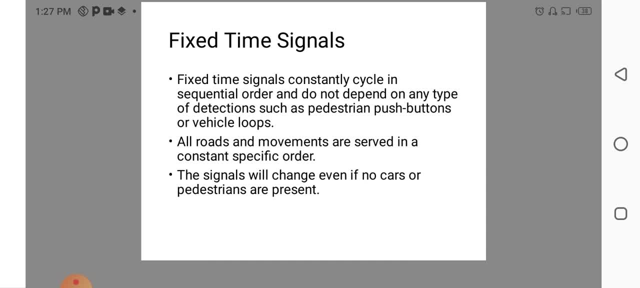 signal. constant traffic signal. fixed time signal. fixed time signal. constant traffic signals. fixed time, fixed time. all total signals are efficiently cycling in sequence order and do not depend upon any type of detections such as pedestrian push-button or vehicle loop. all roads and moments are served in a 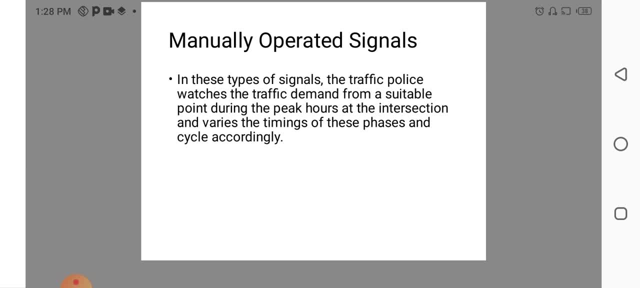 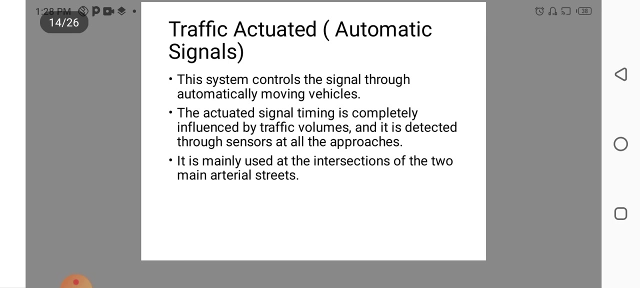 constant specific order. manually operated signals. this manually operated signals are operated by traffic police watches. the traffic light signs on these signals are operated by traffic police watches. the The traffic police watches the traffic demand for a suitable point during the peak hours at the intersection and varies the time on this pace and cycle accordingly. 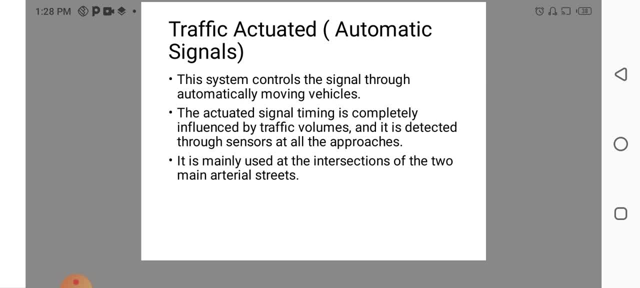 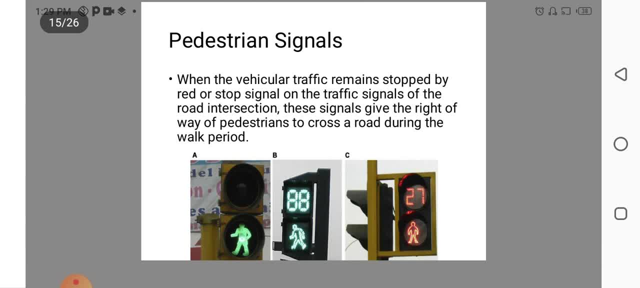 2-2-1,. 2-2-1.. Main address: splits Pedestrian signals When the vehicular traffic remains stopped by the radar stop signal on the traffic signal of the road intersection. the signals give the right of way to pedestrian to cross the road during the work period. 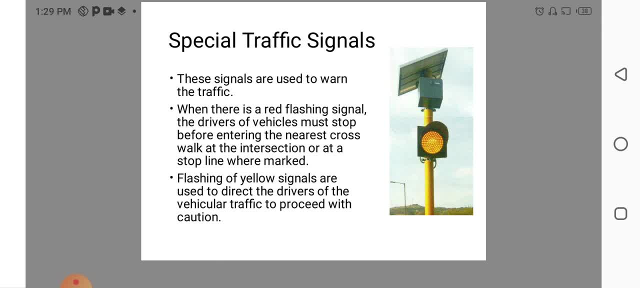 Special traffic signals. These signals are used for one the traffic. When there is a red flashing signal, the driver of the vehicle must stop before entering the nearest crossing walkway, at the intersection or at the stop line, where marked Flash of yellow signals are used to direct the vehicle driver to the next stop. 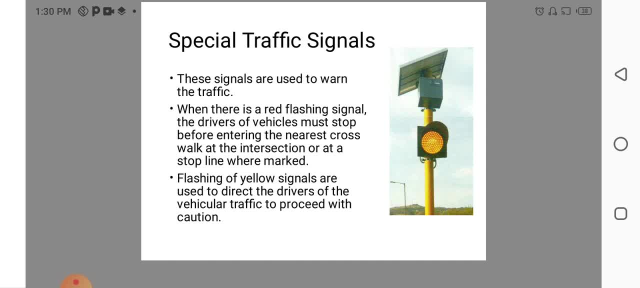 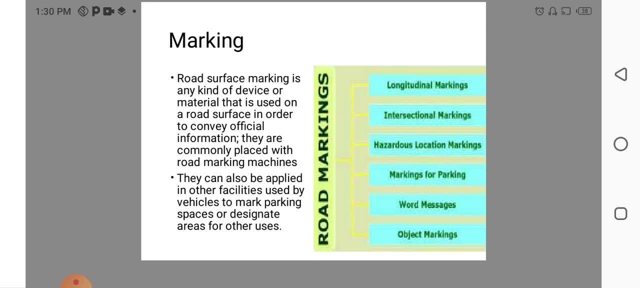 The traffic will stop at the intersection or at the stop line, where marked Flash of yellow signals are used to direct the vehicle driver to the next stop, To proceed with caution. now we can talk about markings. Marking is a kind of device or a material that is used on the road surface in order 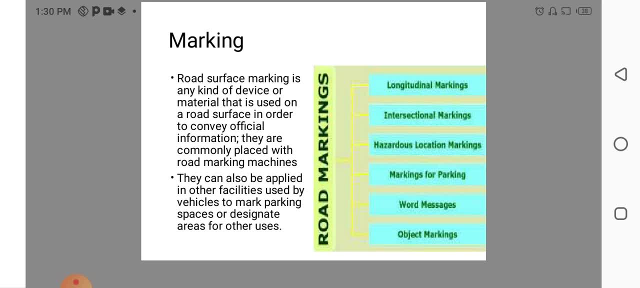 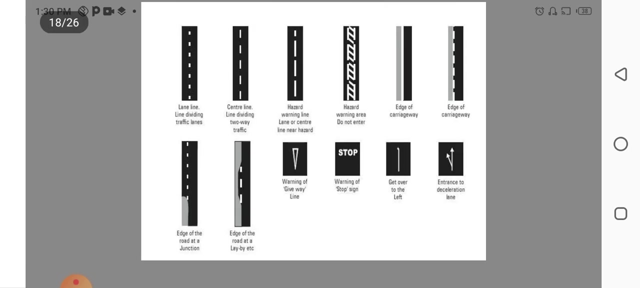 to convey official information. They are commonly placed with road marking machines. Here are some of the markings type: Longitudinal markings, intersectional marking, hazardous location marking, marking wheel for parking word message, object message: you can see some of the marking shown for lane central. 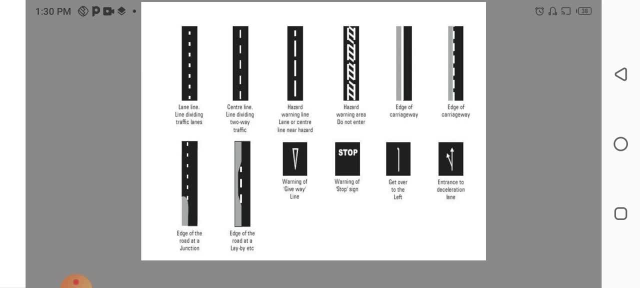 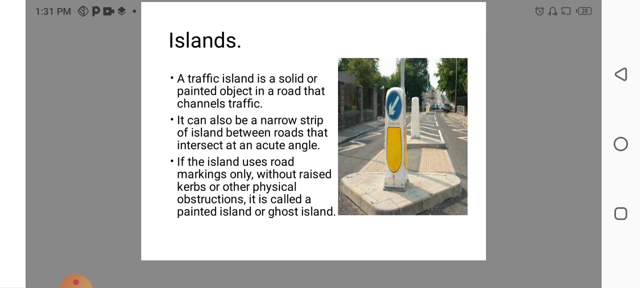 lane, hazardous edge of garage way, etc. Island. Island is a solid or a painted object in the route that channel traffic. It can also be a narrow strip or island between routes that intersect at an acute angle, If the island uses road marking only without raised curve or other physical obstruction. 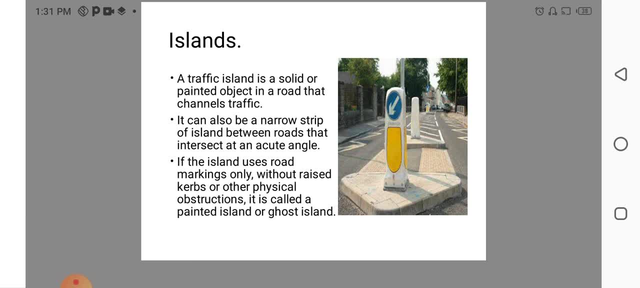 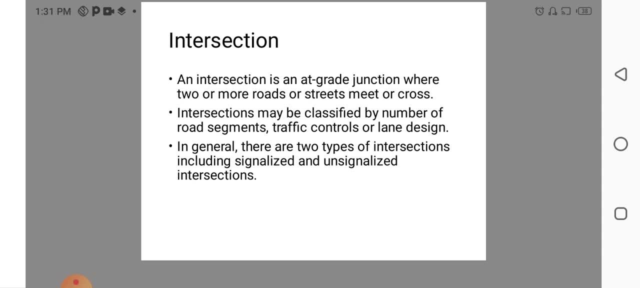 it is a painted island or ghost island. Now, last but not the least, we will be talking about intersection. Intersection is an at-grade junction by two or more roads or a street meet or a crossing. Intersection may be classified by number of road segments, traffic control or a lane design.